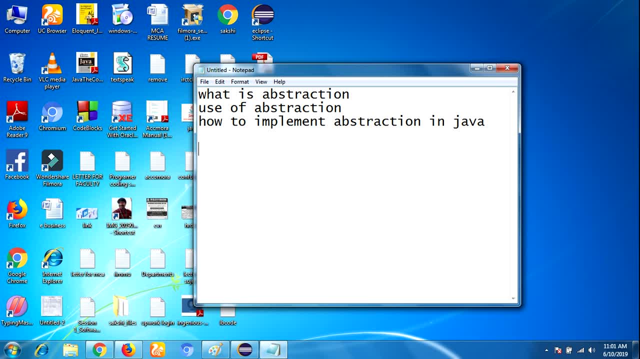 That means exposing the important things to the user. That means exposing the important things to the user And it hides the internal details. So what is the use of abstraction? So it reduces the complexity to the user. So it may be a complex. it is a technical term, technical definition. you may not understand properly. 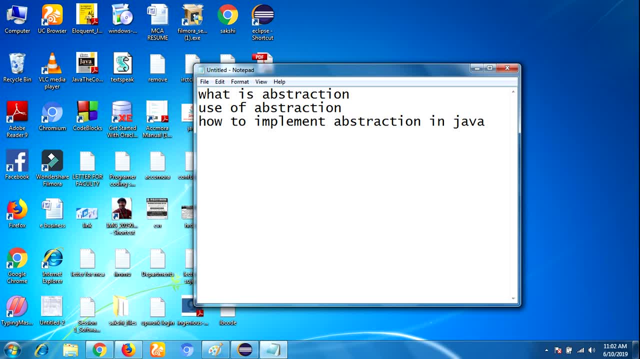 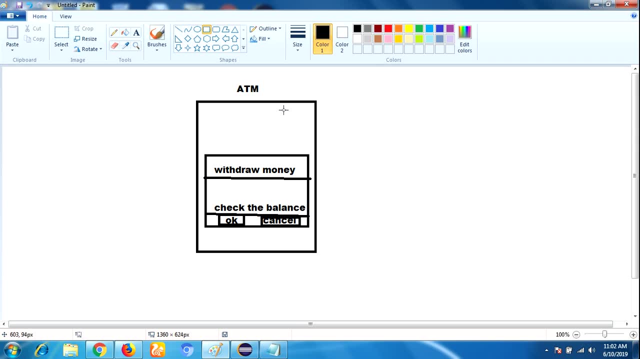 Let me take an example. Consider an ATM machine. Consider an ATM machine. It shows some options like: this is an ATM machine. suppose this is an ATM machine. It has some options like operations: withdraw money, check the balance okay and cancel. 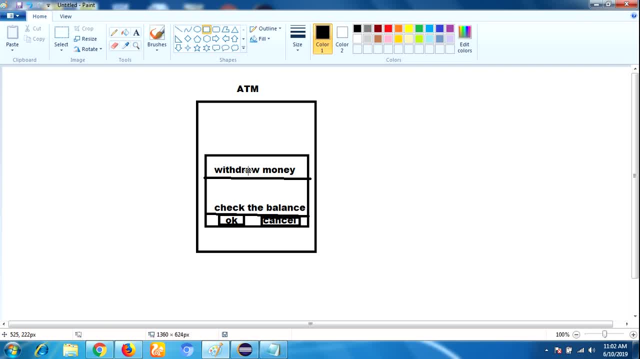 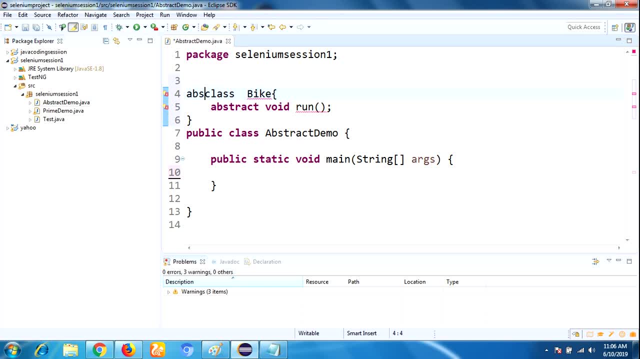 And that's the Tambourine aws. If any of thisη teasing have the use of abstract method and you want to declare it means that, then you want to declare it means that, then you want to declare it means that this is the new abstract Introduction method. 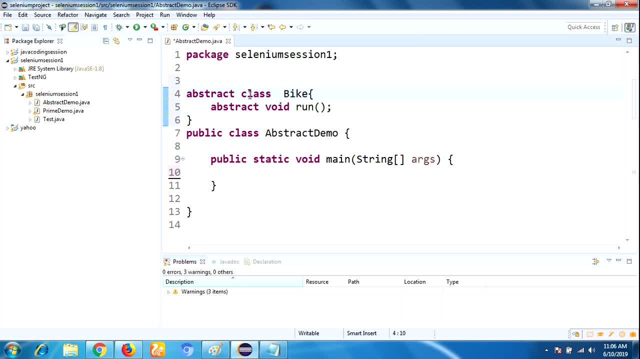 this is the new abstract Introduction method, and this is my new abstract introduction method. that means we have to declare, we have to define abstract keywords. So now, here is the answer, then: how to implement this method Further. to do that, We need to create a new class. 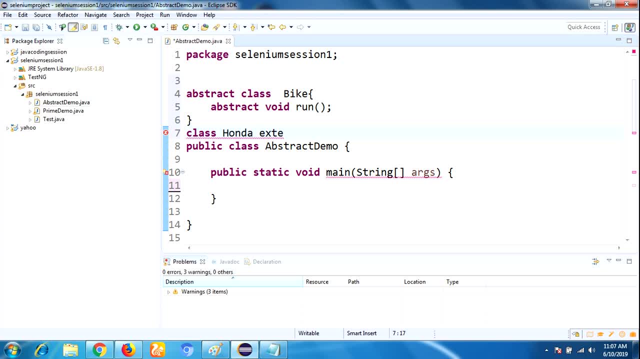 class fonda by using extends the keyword and implementing the method. to implement the method public wide run. ok, and here piso system. so fonda by is running ok. so this is the way to implement abstract method by creating new class and extending the abstract class. ok, then for which class we need to create object? 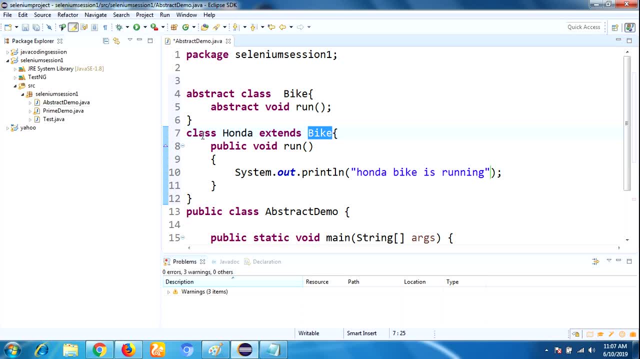 this is abstract class or normal class, ordinary class. we can create this class, we can create the always for normal class only. we cannot instantiate the. that means we cannot create the object for abstract class. ok, for that we need to create the object in main method. so fonda h equal new fonda. 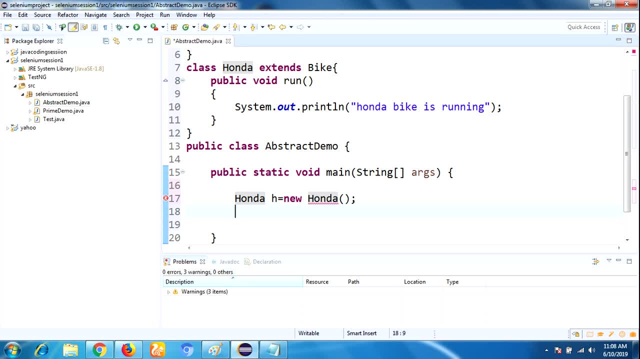 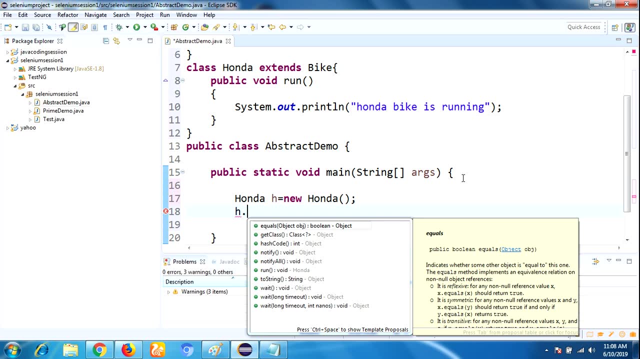 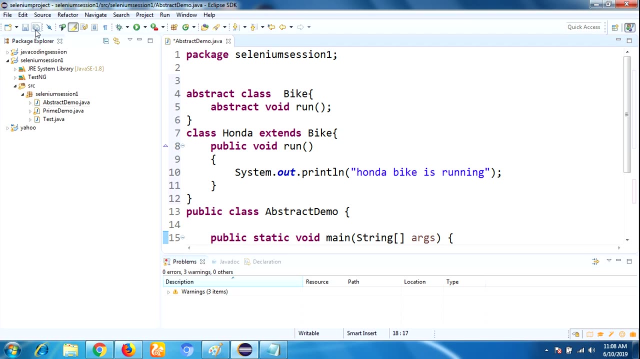 then how you can call that method class method, fonda class method by using object reference name, dot method name. what is the method name here? run? ok, now save the program and run the program. to run the program, click on the run button. see here output. the output will be here: fonda by is running. 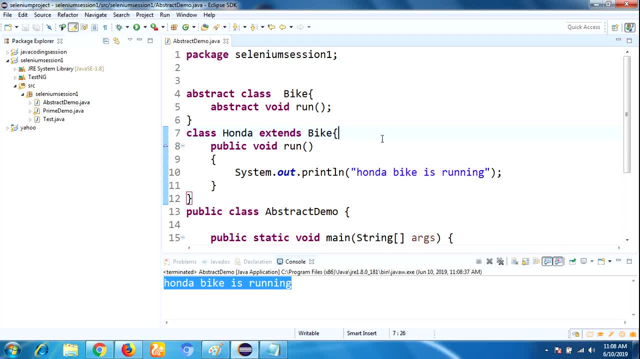 so this is the way to implement abstraction: by using abstract class. so remember these points, guys: whenever the class having abstract method, the class must be doing abstract method, the class must be declared with the abstract keyword right. so we need to implement those methods by creating new class. 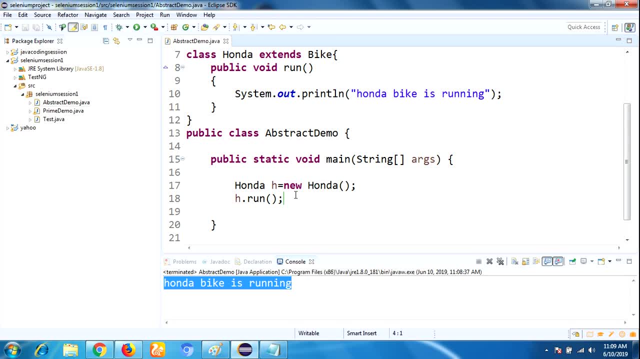 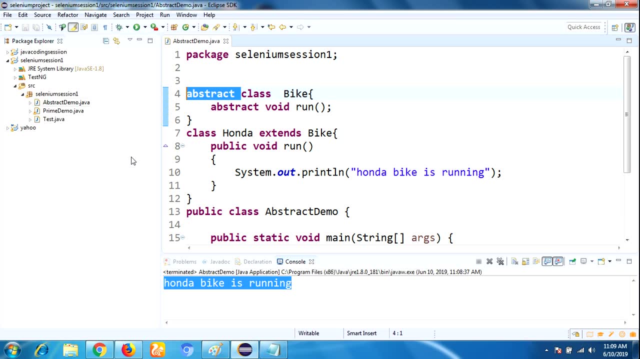 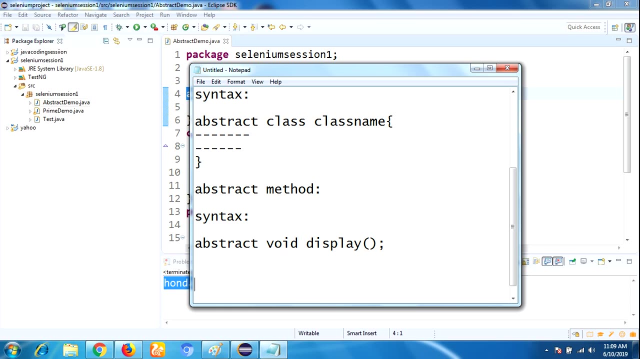 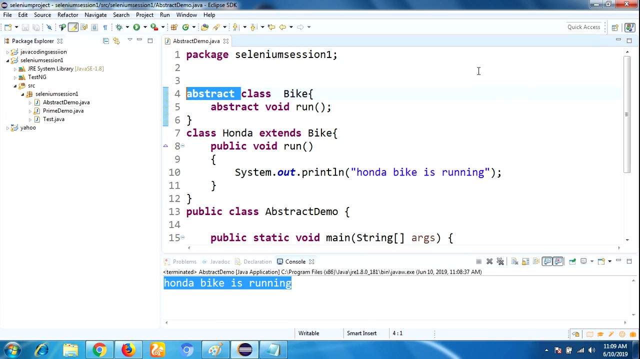 right, so this is the process to create abstract class. ok, so then, how to implement, how to achieve abstraction by using interface here, interface means what is the definition of interface? interface means it is a hundred percent abstract method. all are abstract methods only in interface, whereas in abstraction, in abstract class. 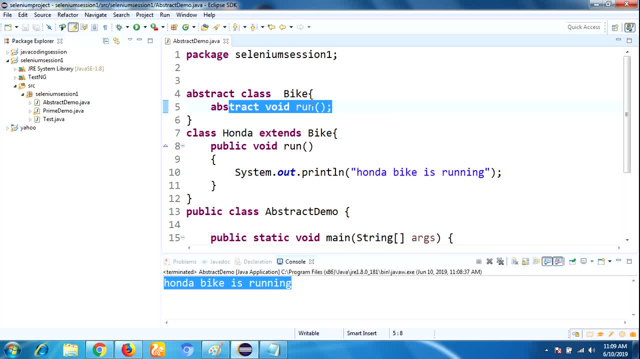 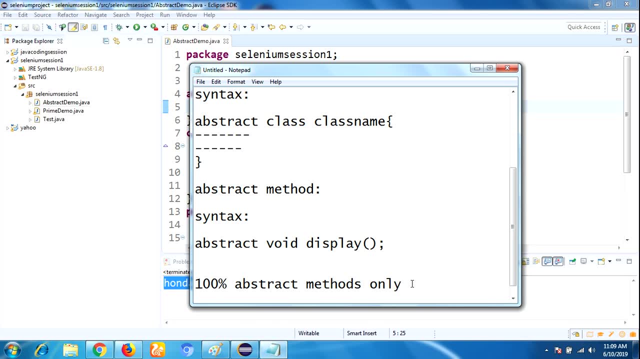 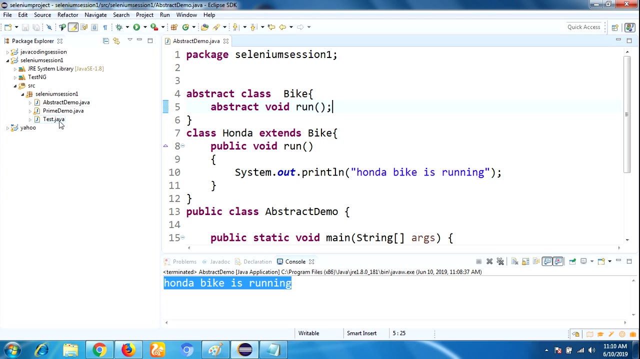 whether you create abstract methods and concrete method as well, no problem at all. but in interface, all are having abstract methods only. ok, so how to achieve abstraction by using interface? so let me, let me give an example, then you can clearly understand. I have already created one test class here. 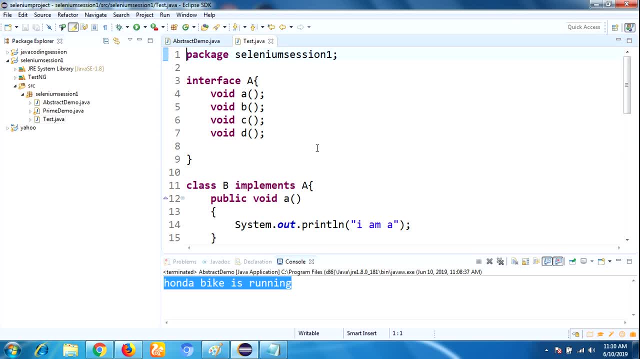 see, here I am taking one class, so the class name is this: ok, so I have taken here interface name as a and I declared I defined four abstract methods. by default, compiler will take the all are abstract methods only within the interface. ok, whether you are declaring or not, no matter. 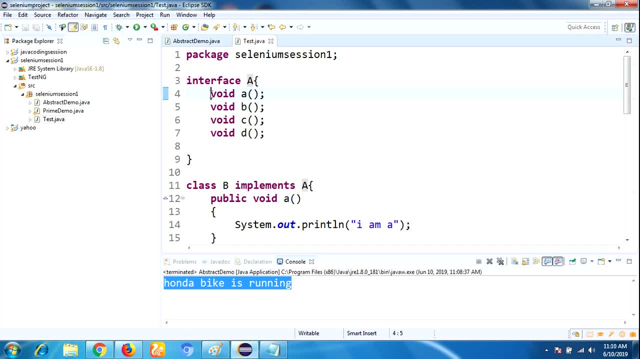 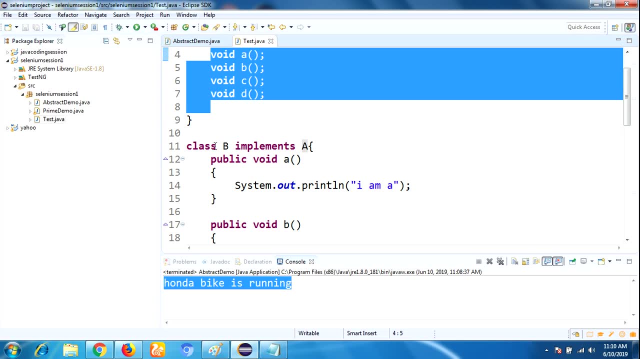 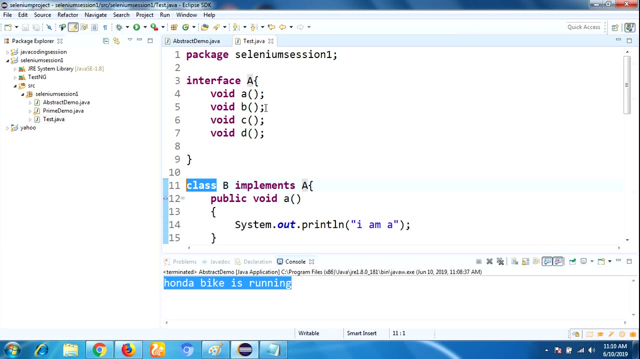 but it is considered all methods are abstract methods only. ok, so we need to implement these methods by creating, by implementing class, new class. I am taking on b class and implements the a. ok, so all abstract methods are I implement. here I am a and here I am giving b. 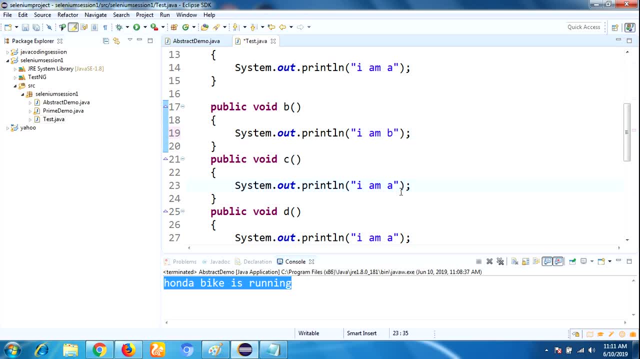 and here I am giving c and here I am giving d, and then I am creating the object for which class class b- see here. ok, new, I am creating object for class b. ok, here I am taking just reference. this is the. this is the actual procedure. is there in java. 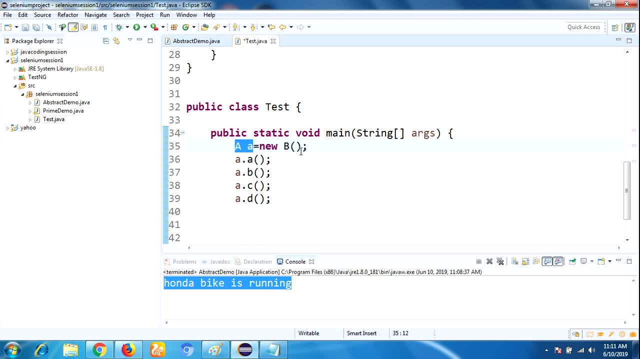 you can just to give the reference to the interface. ok, but we are actually creating the object for b class here. but by what? we are using reference of the a interface. ok. so by using reference we are calling all the methods, whatever available in this method. ok, so because these all methods are implemented in which class? 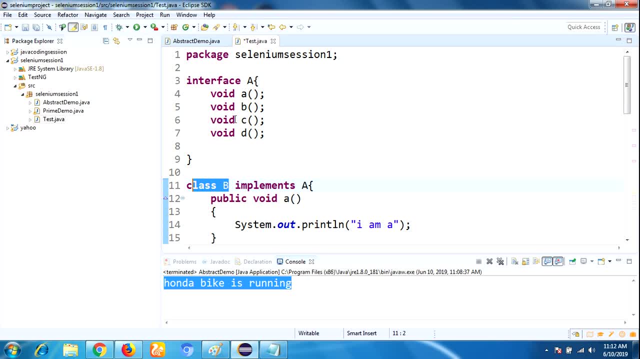 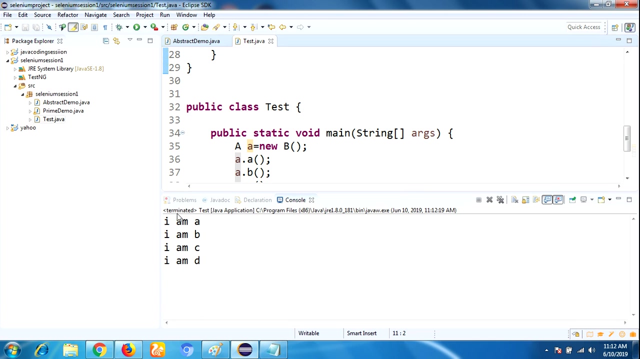 class b. that's why we inherited all these methods in this class b. ok, that's why this class having all the methods here, ok, so let me check, let me try to explore this program, save this program and run this program. see the output. see the output. so I am a and b and m, c, d. 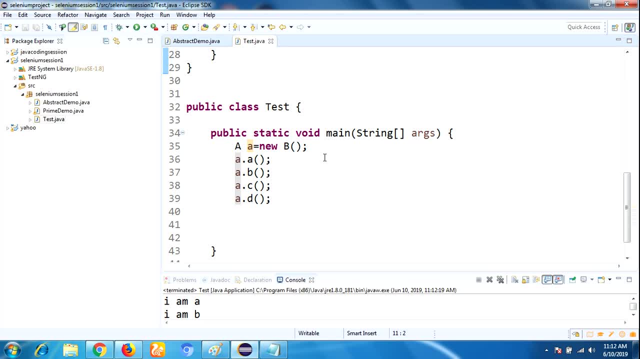 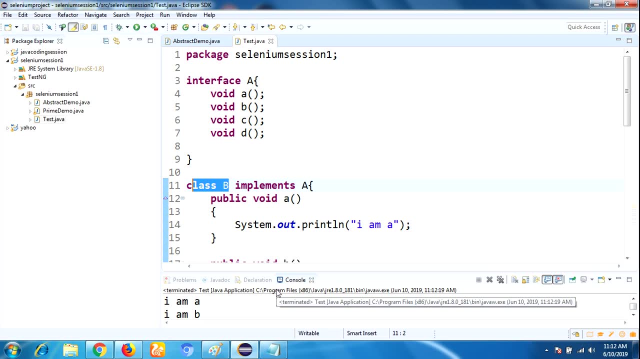 ok, so this is the way we can implement the abstraction- by using interface as well. ok, so we need to. you need to remember some points about abstraction. the first point is: in java, you cannot create instance of abstract class using new operator. it is a compile time error. 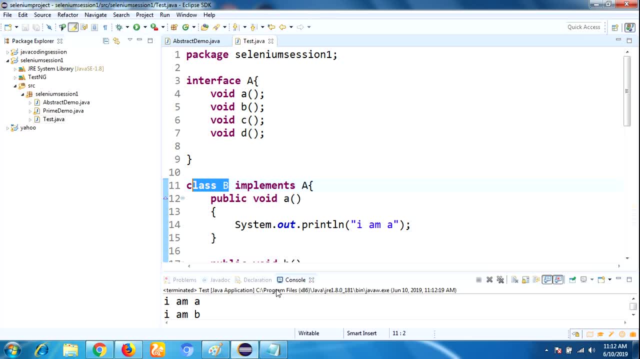 ok. so the second thing you must remember: abstract is a keyword in java which can be used with both class and method. we are using abstract keyword for class and method, already shown in, already shown in in our example program, see here. for class also, we are having abstract. 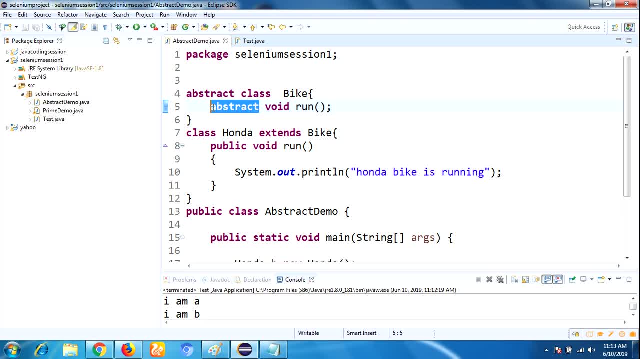 and method. also we are using abstract keyword. ok, so abstract class can contain both abstract methods and concrete methods. we can also declare: this is the abstract method. we can also declare some concrete methods also, no problem at all. ok, so abstract method means. what is the abstract method means? 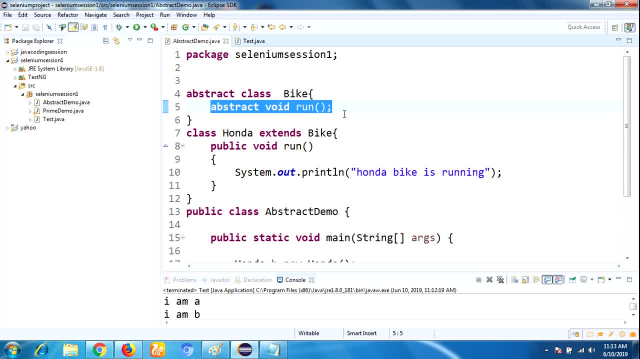 it doesn't have any body, just declaration only. we are just declaring the method, we don't have any method body. ok, so the third thing is: a class automatically becomes abstract class when any of its method declared as abstract. see here, whenever we are declaring any abstract method. 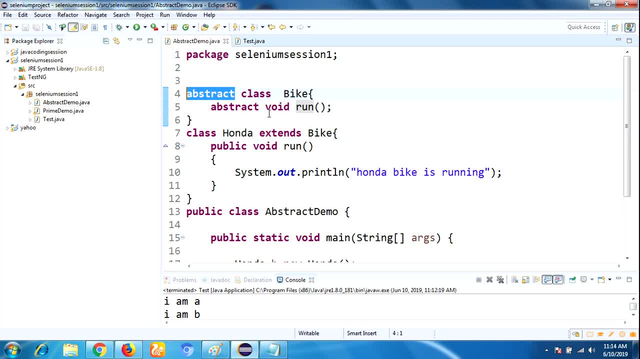 the class must be declared as abstract. i already discussed this point, so these are the things you must remember while defining or declaring the abstract class. ok, so i hope you are understanding this concept. so thank you for watching.